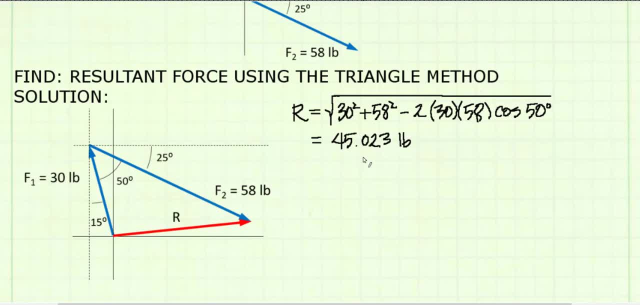 in pounds And I get 45.023 pounds. To three significant figures, R is 45.0 pounds. I can now use the law of sines to find the other interior angles in my triangle. The only other angle I need is angle B, but for academic reasons I'm first going to find. 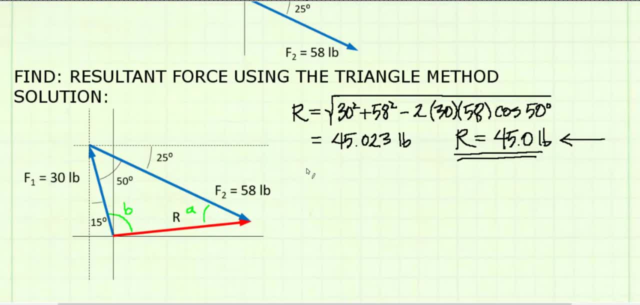 angle A. using the law of sines To find angle a, I will take the sine of A divided by the opposite side of the triangle. To find angle a, I will take the sine of A divided by the opposite side of the triangle. 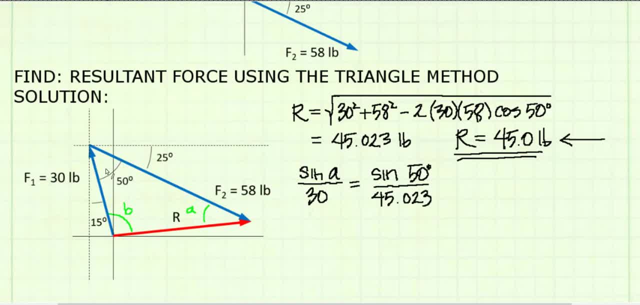 which is 30 pounds, is equal to the sine of 50 degrees divided by its opposite side, which is the resultant force 45.023 pounds. I find that A is equal to 30.693 degrees. Now I will do the same for angle B. 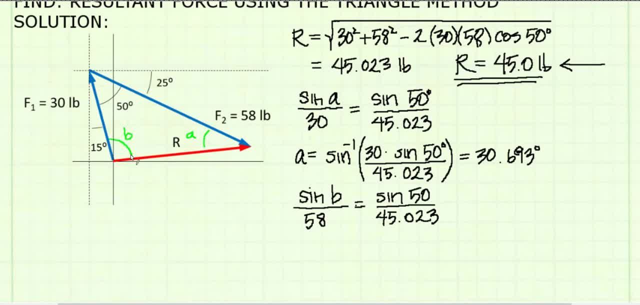 To find angle B, I will take the sine of angle B divided by the length of the opposite side- 58 pounds- and set it equal to the sine of 50 degrees divided by its opposite side, 45.023 pounds. 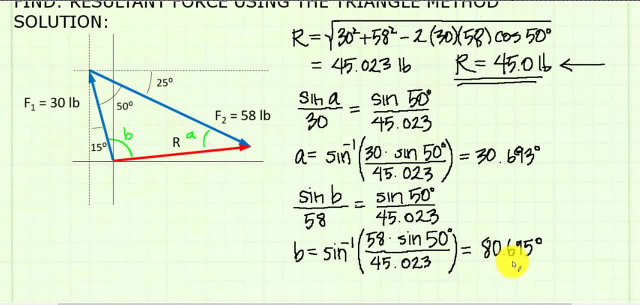 And solving for angle B, I get 80.693.. Now if I look over at angle B, I'm a little surprised because I tried to draw these vectors to scale and it seems like that angle is more than 90 degrees. so this answer is a little concerning to me. 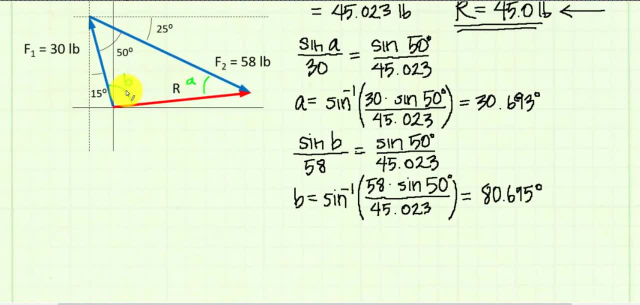 In fact we can check it, because the angle A plus B, plus the 50 degrees for the third angle should all add up to 180 degrees. Let's check it out. Well, my suspicions are right. Something's gone wrong. My three angles do not add up to 180 degrees. 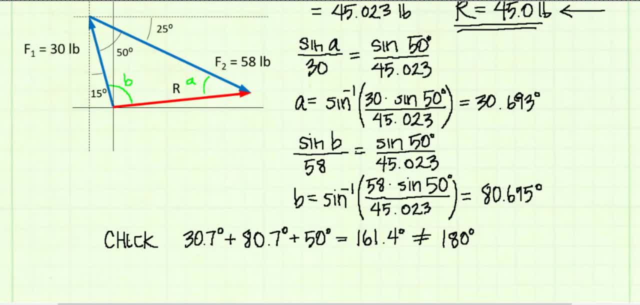 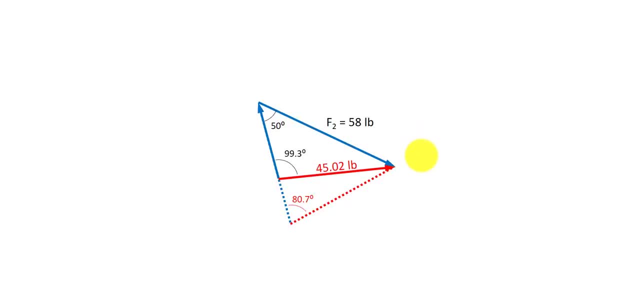 There is no math error. This has to do with a little quirk when using the law of sines. This is what happened when I did the calculation. The values that I put into the law of sines equation used this side, the resultant force side. 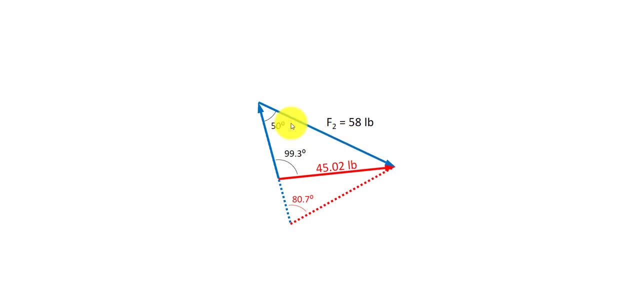 the force F2 side and this angle. So a side, a side and an angle. Sometimes when using law of sines, in these conditions there are actually two solutions to the answer, And I was unlucky and got the wrong solution. 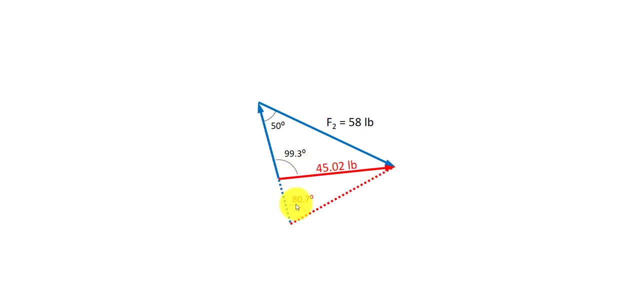 The value that my calculator returned is the angle 80.7, as shown by these dotted lines. Now, this red dotted line has the same length- 45.02.. The force F2 has the same length- 58 pounds, and the angle 50 was unchanged. 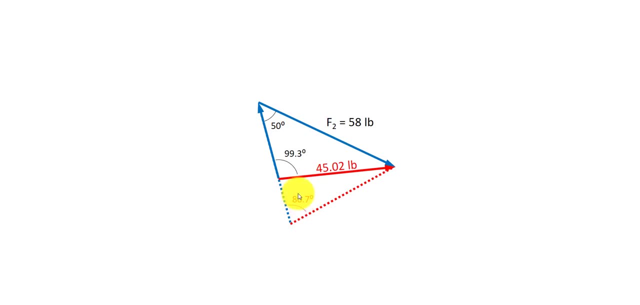 But you can see there are two solutions. My calculator gave me 80.7, but the correct answer is actually 99.3 degrees. This doesn't happen very often, but it can happen and it's good to be aware of it. 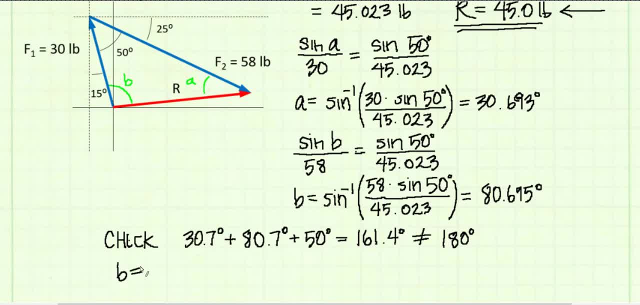 So what do we do? Well, the correct angle for B is 180 degrees minus the value we got above Calculator. Calculating it gives us 99.305 degrees and that looks better. Angle B looks like it's more than 90 degrees and 99.3 seems about right. 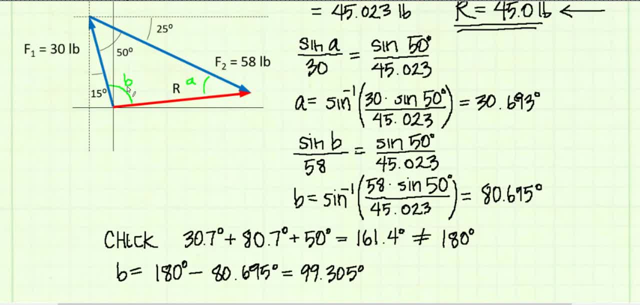 So here's a good lesson from this: Draw your vector diagrams to scale so you can recognize if you have an error or at least have a better chance of recognizing it. If we did a quick check and added 30.7 degrees to 99.3 degrees to 50 degrees are three angles. 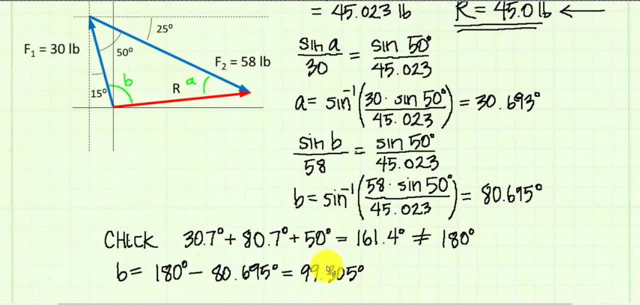 that would indeed Equal 180 degrees. Now we still need to find the direction of our resultant force vector. I'm going to label it like this in the figure and call that angle theta. I'm going to use angle B to find theta. 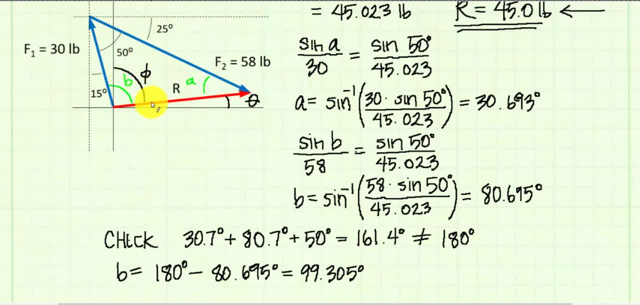 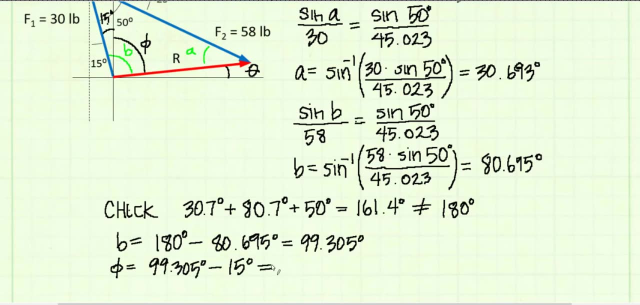 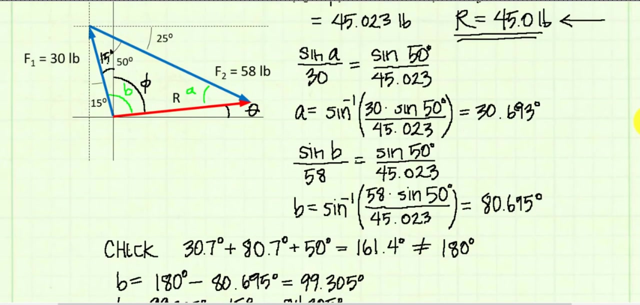 I'm going to call this angle that I've drawn here as angle phi, and that's going to be equal to angle B, minus this interior angle, which is 15 degrees. I get that phi is equal to 84.305 degrees. And now, looking at the figure one more time,